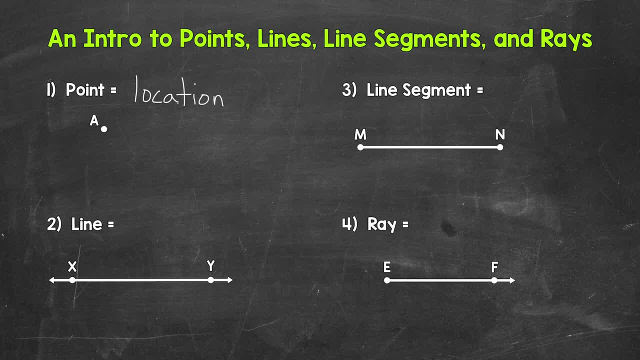 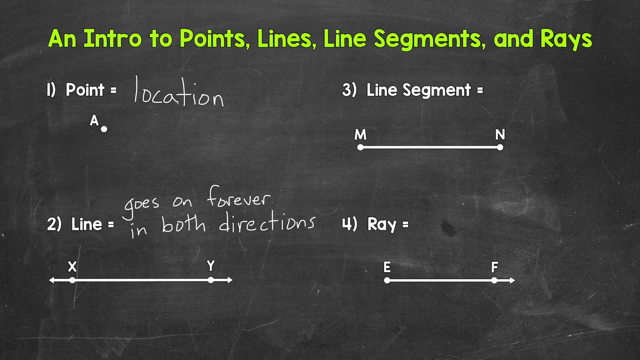 directions. So, in other words, lines extend infinitely Both directions. So let's put: goes on forever in both directions. for our notes And for our example, we have line x, y. The arrows show that the line extends infinitely in both directions. Now, as far as how we're going to do this, we're going to do it in both directions. 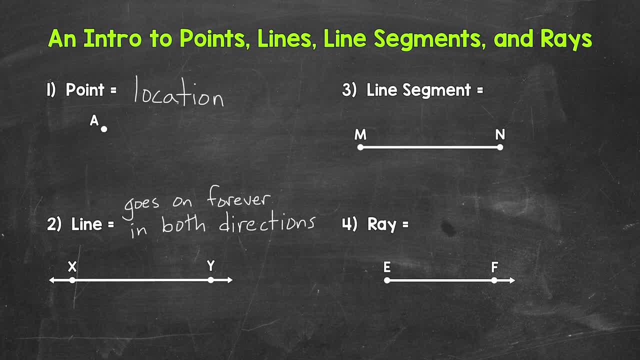 How to name a line. That's something we will cover in another section. But again, for that example, we have line x, y and those arrows show that the line goes on forever in both directions. Let's move on to line segments. A line segment has two end points. They have a starting and 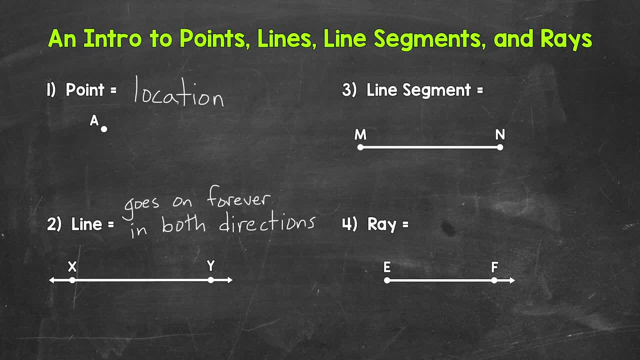 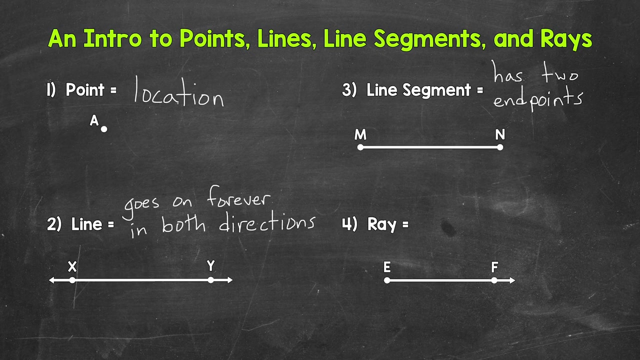 stopping point, so to speak. A line segment can be measured. They don't go on forever. So let's put as two end points for our notes here. For our example, we have line segment m- n. That line segment stops at point m and stops at point n. Those are the two end points And we will go into 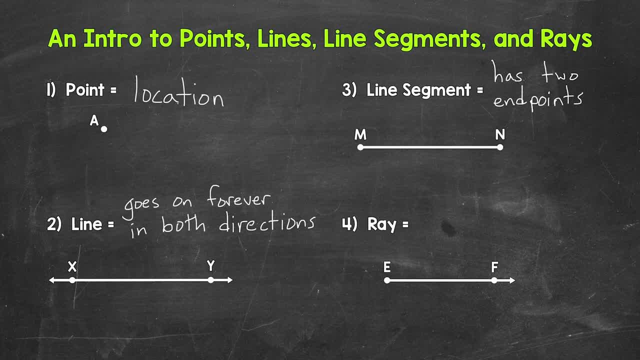 naming line segments in another section. Lastly, we have rays Now. a ray has an end point and then goes on forever. So let's move on to line segments. A line segment has two end points. They have a on forever in one direction, So it extends infinitely in one direction. And I always 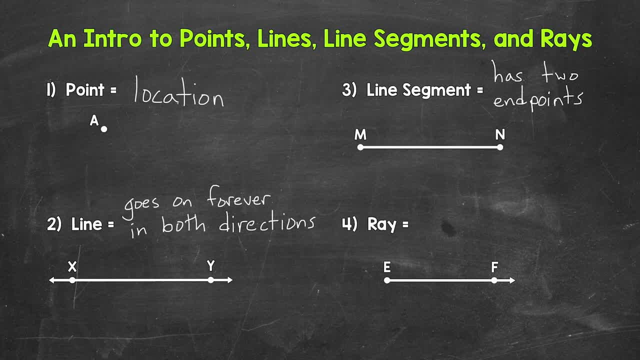 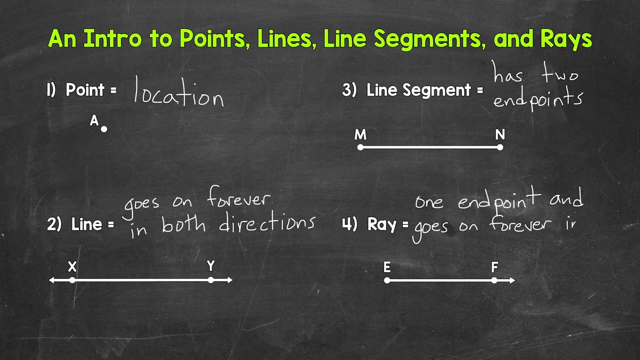 like to think of a ray like a ray of sunshine: The sun is the end point and then the ray goes from there. So and end point, and then goes on forever in one direction. So for our notes, let's put one end point and goes on forever in one direction. And for our example, we have ray EF.